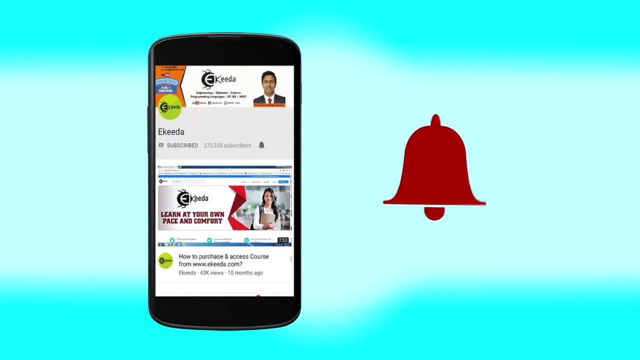 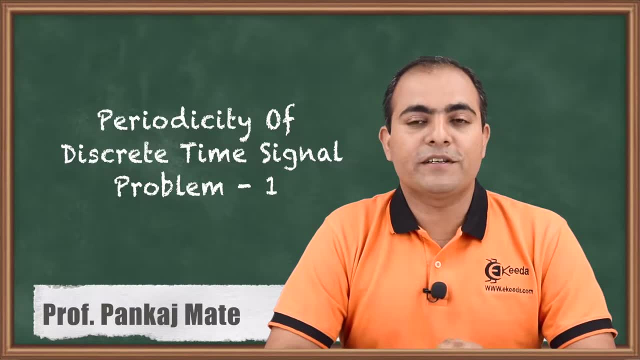 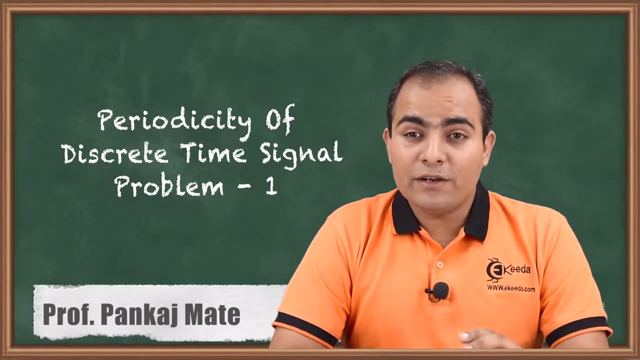 Click the bell icon to get latest videos from eKIDA. Hello, friends, and today we are going to solve a numerical which is based on periodicity of discrete time signal, and the problem is problem number one. Now, what is important? Basically, we want a value of period, that is, a number of samples value, but that value must be in. 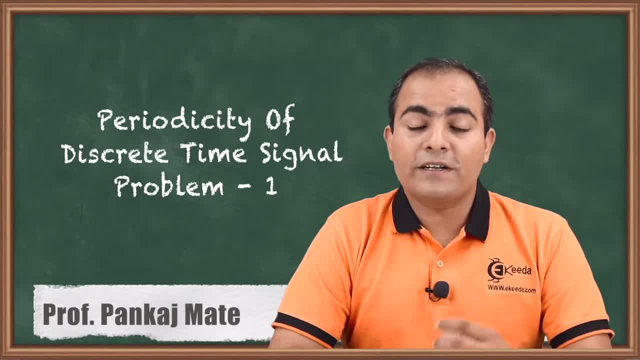 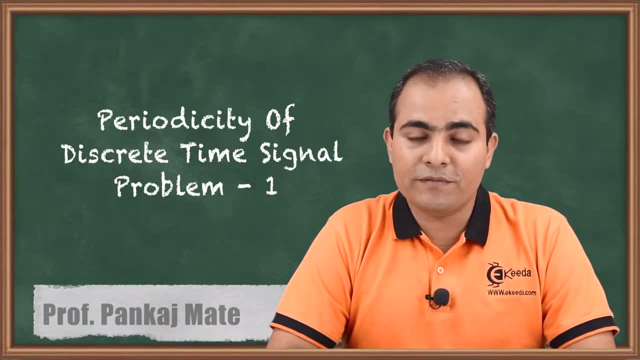 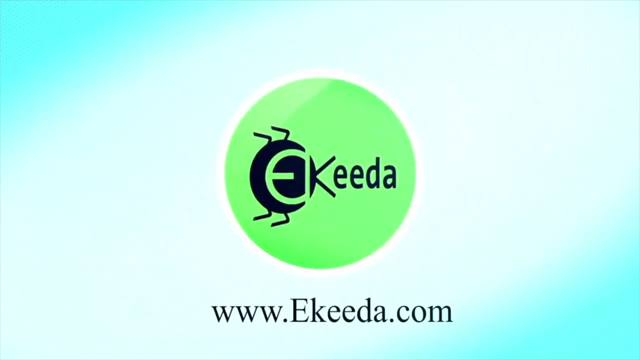 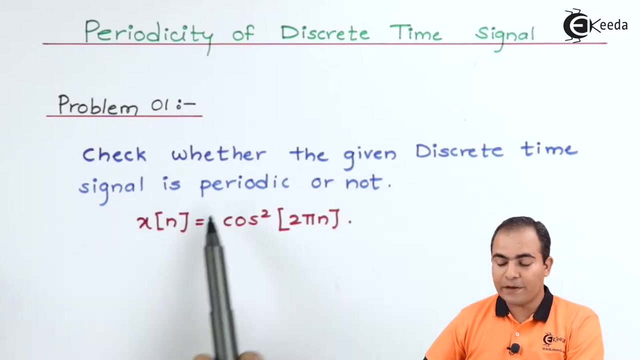 a rational format. How to obtain that rational format and how to obtain the period value that I will show you from this numerical. So let us start with the problem number one. So, problem number one: Check whether the given discrete time signal is periodic or 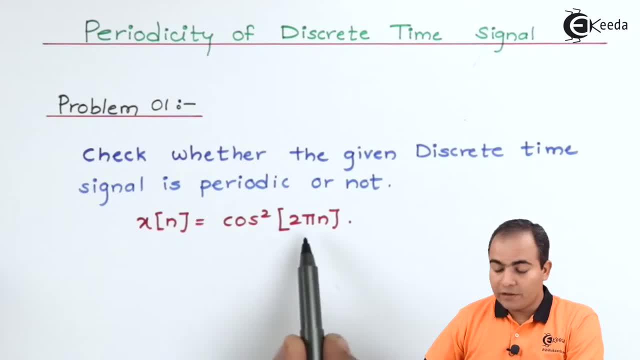 not Now where you will find out the period Over here, Because in many of the questions or in many of the standard equations, we have seen or we have studied one formula, and that formula is a cos of omega n and from this omega you can get the value. 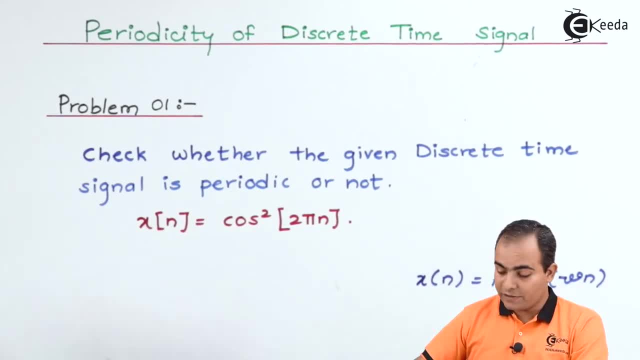 of total number of samples. Now, first of all we will see what is asked. x of n is equal to cos square 2 pi n. Now we want to function in only cos, but here question is given in cos square n, So we can use. 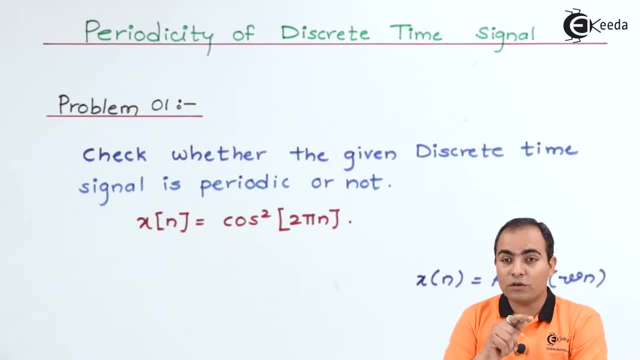 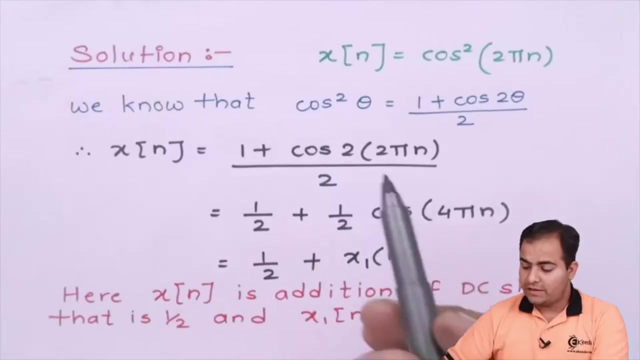 one formula that is cos square theta is nothing but 1 plus cos 2 theta divided by 2, where my theta value is 2 pi n. So I will show you how to solve this question and how to obtain the total number of samples, that is, how to find out the given function is periodic or not. Let us see In this: 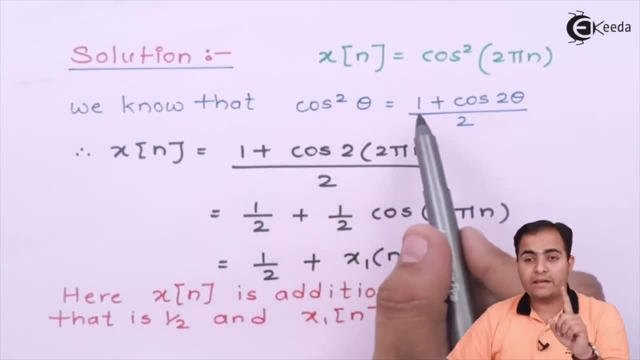 example, we have got 1 minus cos square theta by 2.. The sin square theta is 1 minus cos, 2 theta by 2.. You should know the basic formula is related to cos and sin and it is necessary while solving the numericals related to energy power or a periodic or non-periodic, or if 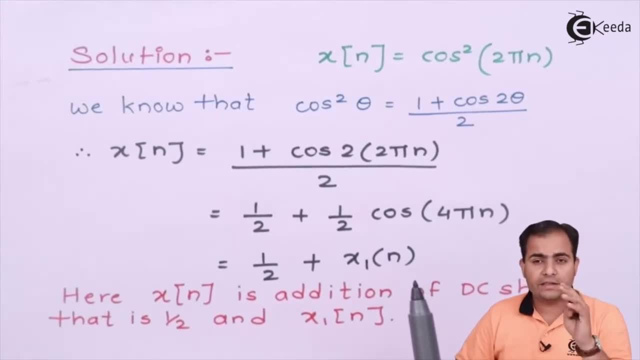 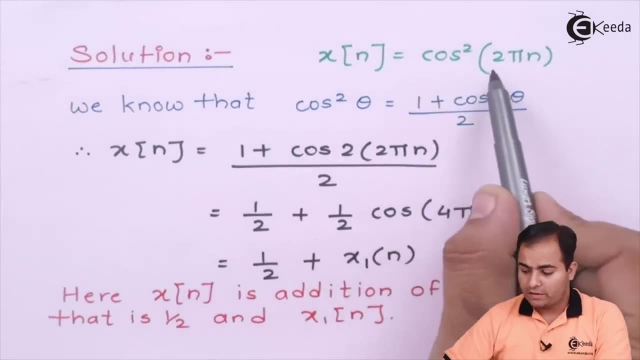 numericals is related in a encounters in a Laplace transform, z transform and the Fourier series. So now come to the point. We will use this formula in our question. So my theta is 2 pi n. So I have just substituted for the theta and I will now try to find out the. 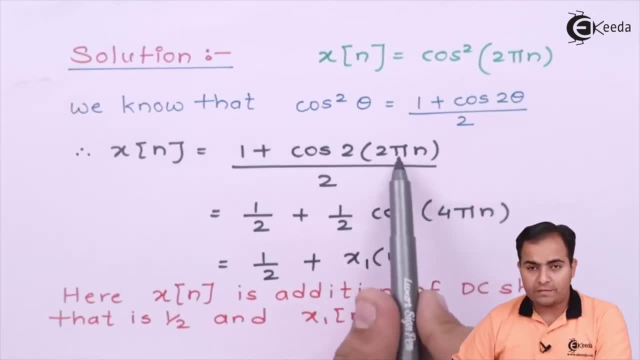 solution. Now we see our solution as follows. What we will do is we will solve this formula in our question. So my theta is 2 pi n. So I have just substituted the theta, that is 2 pi n, in my formula and I am going to change this base. like we know that a plus b by 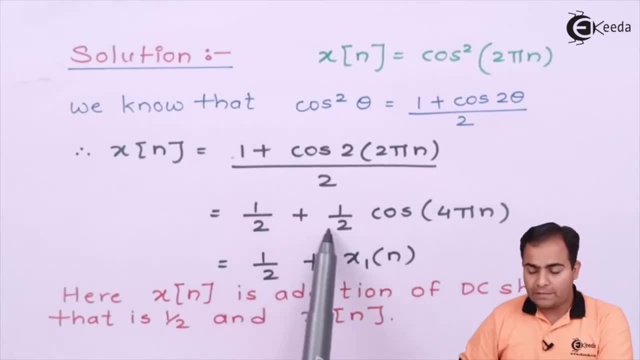 2 can be divided by a by 2 plus b by 2.. So, after separating the base, what you can say that you will get a half, and I have consider this is my x of n. this whole part is my x of n. Now, what is half? 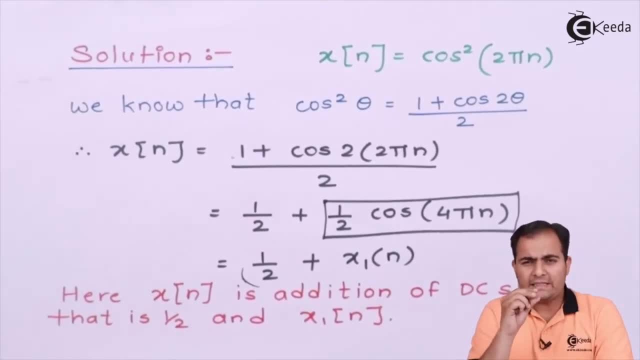 what do you mean by half? half is nothing, but 1 dc amplitude is added in x of n. you can say that when dc amplitude is added in x, 1 of n. So after adding a dc shift or dc amplitude, the function will not get affected. whether it is periodic or non-periodic, it will follow the same sequences. 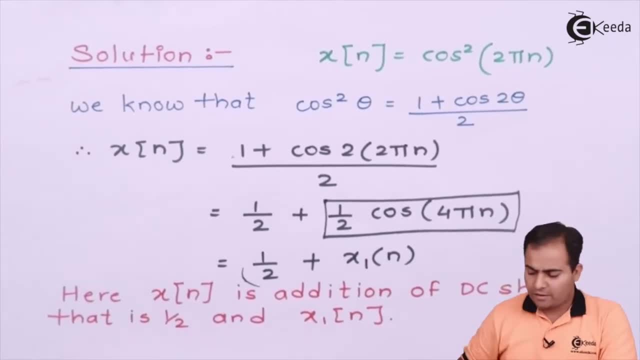 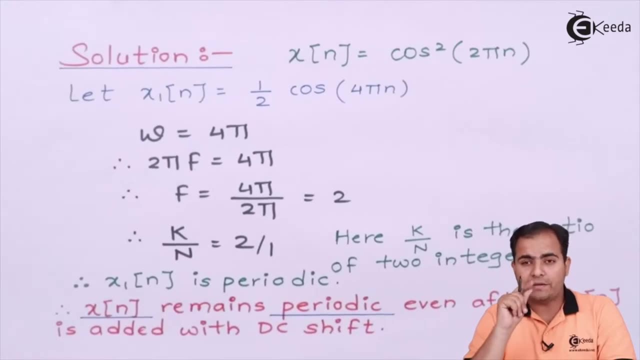 after adding a dc shift. So half does not matter at all. but what about x of n? whether x of n is periodic or not, we will see. Now we will see the periodicity of x of n, because total x of n is completely depends on x 1 of n. because, as I said earlier, we will see the periodicity of x of n. 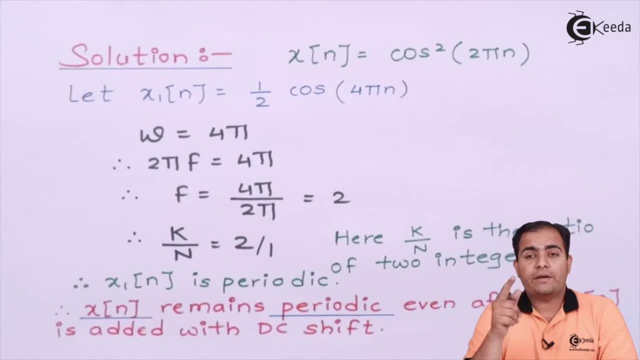 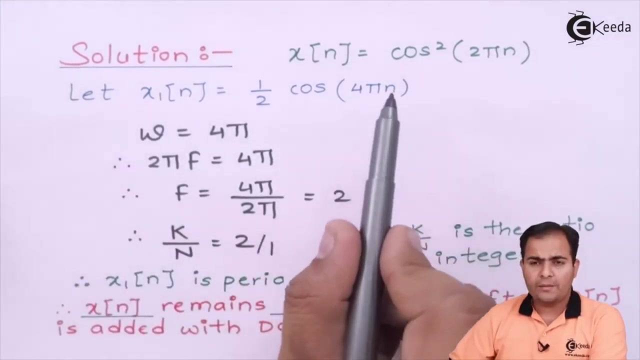 because, as I told you earlier, dc shift will not affect the periodicity or non-periodicity. only. the thing is x of n is completely depends on x 1 of n. So let us see x 1 of n is periodic or not. Now let us say my x 1 of n is half of cos of 4 pi n. I am going to compare the frequency of cos 4. 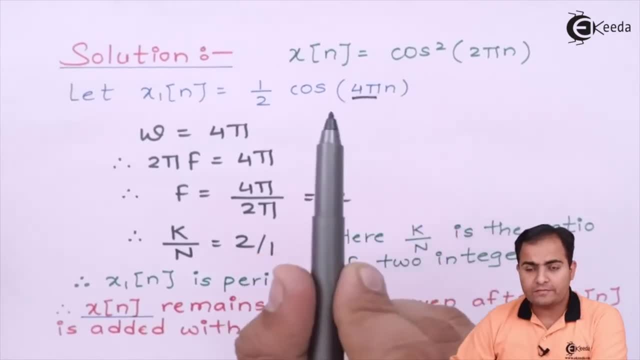 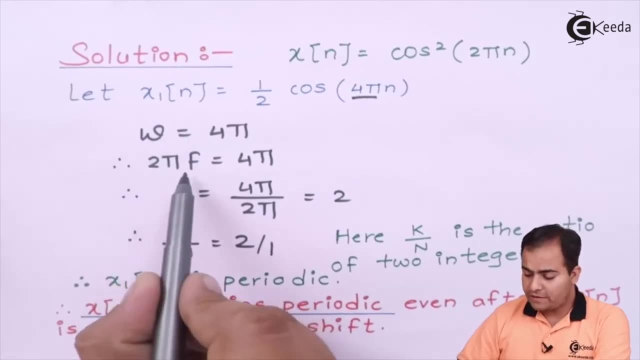 pi n. So this is my frequency omega. I have just compared this omega. we know that omega is 2 pi, So f is nothing. but I am going to shift this 2 pi on left hand side. So 4 pi by 2 pi is t2.. Now 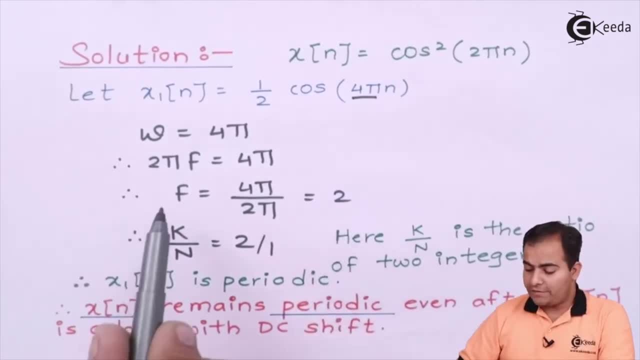 in frequency. in discrete part this frequency is represented by k, by n, where n is the period and the k is the number of cycles. So you can say that here the value is 2, this value is 2.. So I can write this 2 as 2 by 1 also, or simply you can keep it as it is. But now look at here: 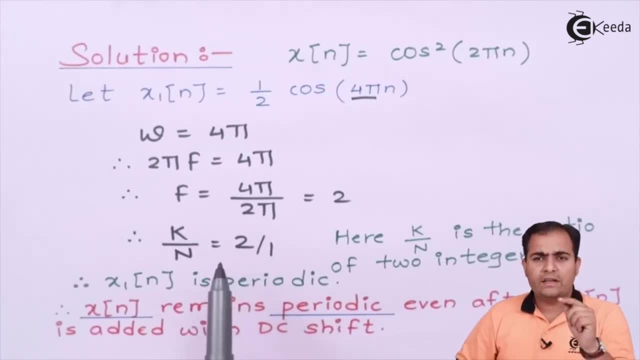 value 2 is perfectly rational. or you can say, a perfect combination of two integer. That's why I have divided it by 1.. If you divide it by 1, then also it is fine. If not, then also it is fine. Just one thing is necessary: Whatever result will come, this result should always have the